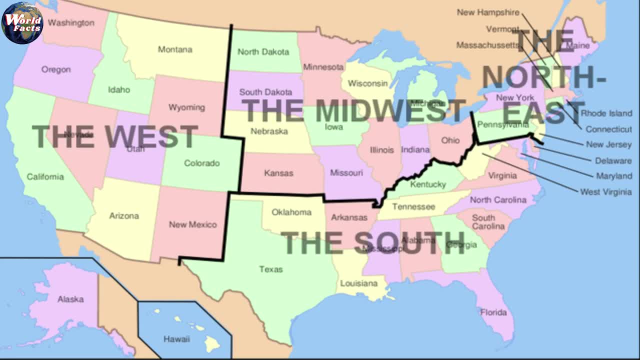 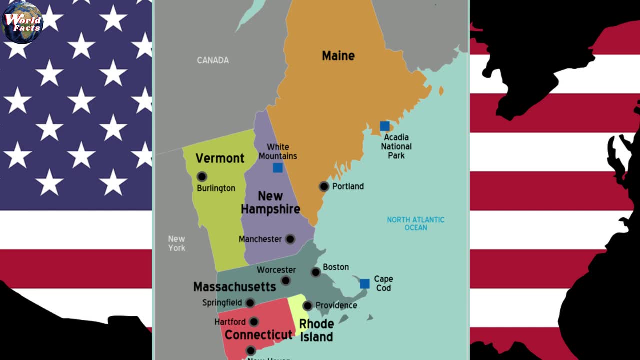 New England, the Mid-Atlantic, the South, the Southwest, the Midwest and the West. European settlers from the West, Southwest and Midwest came to New England to seek religious freedom. The population is diverse. people from all over the world seek shelter and a better life New England, the Mid-Atlantic, the South, the Southwest, the Midwest and the West. European settlers from the West, Southwest and Midwest came to New England to seek religious freedom. these states are connecticut, maine, massachusetts, new hampshire, rhode island and vermont. the mid-atlantic region includes delaware, maryland, new jersey, new york, pennsylvania and washington dc. these industrial areas attracted millions of european immigrants and gave birth to some of the largest cities on the east coast: new york, baltimore and philadelphia. to the south of the states of alabama, arkansas, florida, georgia, kentucky, louisiana, mississippi, north carolina, south carolina, tennessee, virginia and west virginia, the midwest is called the bread. 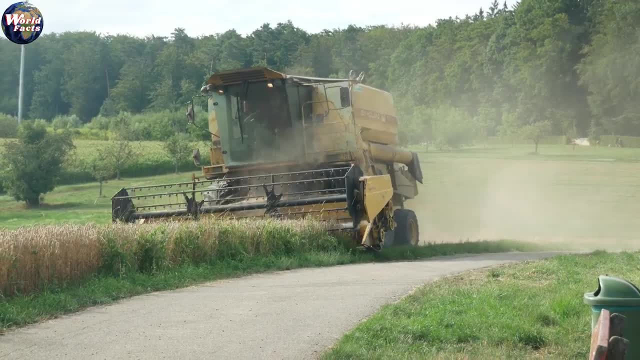 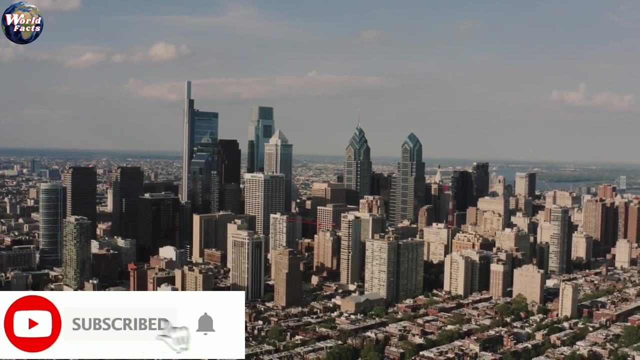 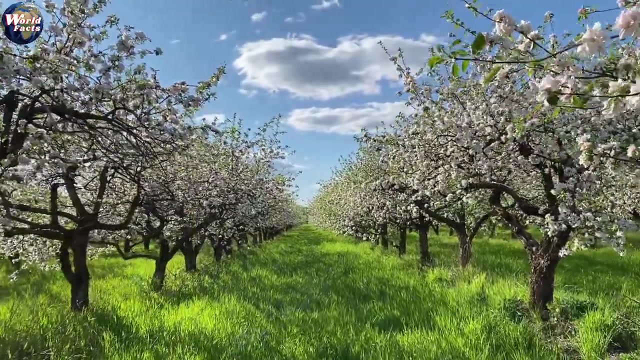 basket of the nation, as it is home to the country's agricultural base. the region includes illinois, indiana, iowa, kansas, michigan, minnesota, missouri, nebraska, north dakota, ohio, south dakota and wisconsin. the southwest is a beautiful grassland and desert landscape: arizona, new mexico, oklahoma and texas. 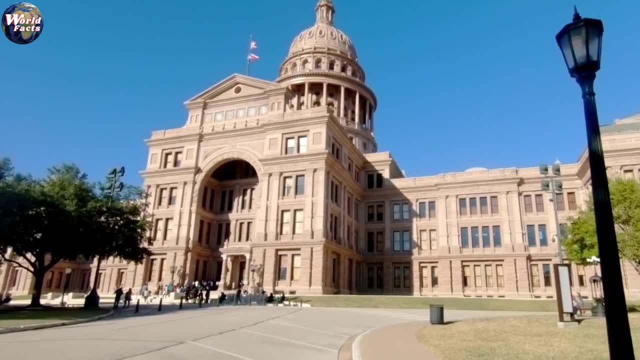 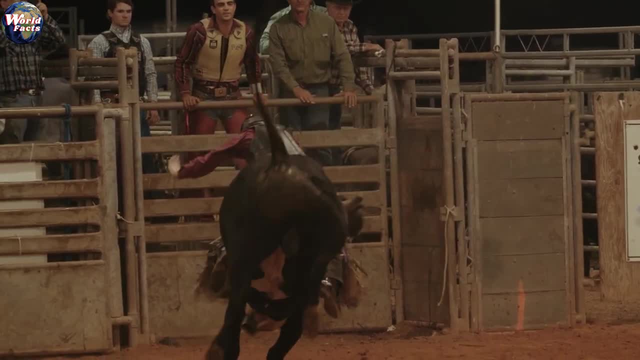 are considered to be the southwest, with some of the greatest natural wonders in the world, such as the grand canyon and carlsbad caverns. the west is the home of rolling plains and cowboys, and a symbol of american innovation. it is diverse, from endless wilderness to arid deserts. 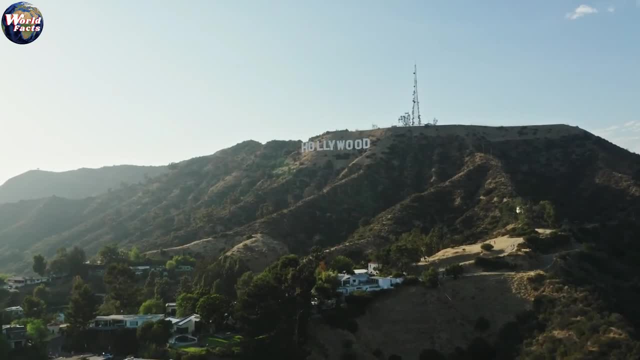 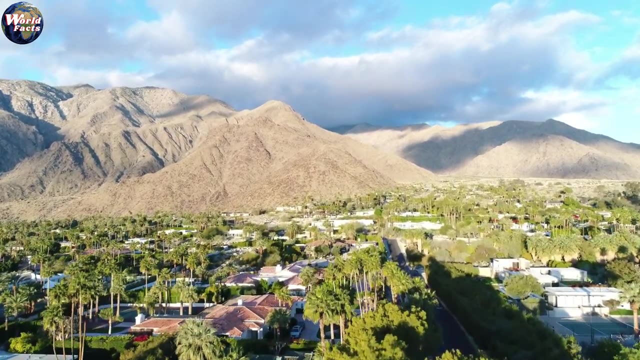 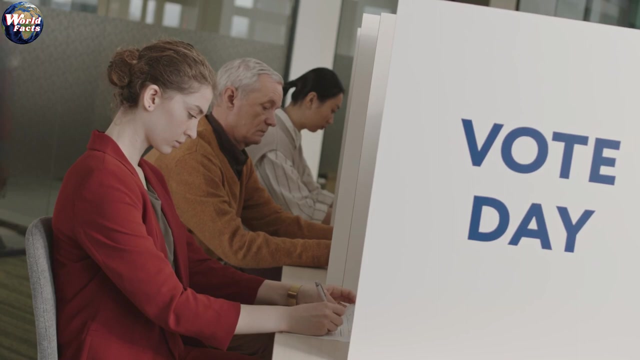 coral reefs and arctic tundra, from hollywood to yellowstone park. these include alaska, colorado, california, hawaii, idaho, montana, nevada, oregon, utah, washington and wyoming. citizens over the age of 18 elect the president and vice president of the united states every. 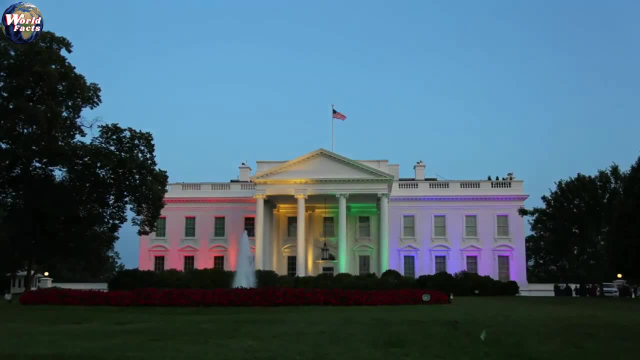 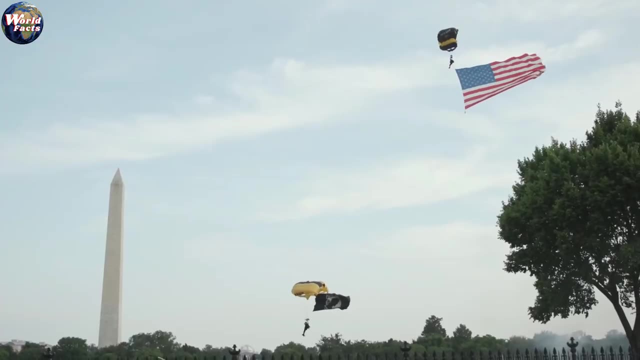 four years. the president lives in the white house in washington dc. the congress has two houses: the senate and the house of representatives. there are 100 senators, two from each of the 50 states, each for a six-year term. 435 of the senate and the house of representatives are elected from each of the 50 states, each for a six-year term. 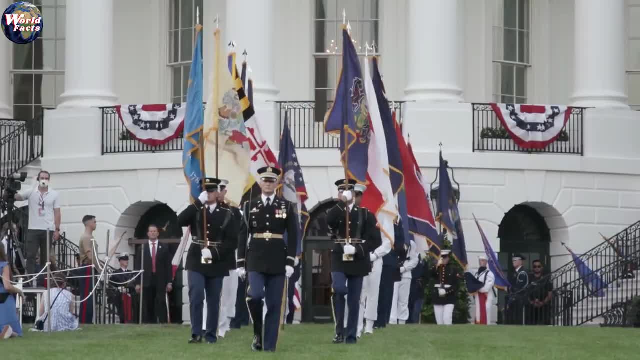 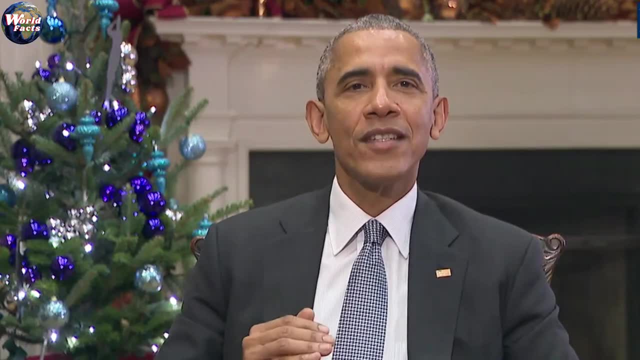 counselors are elected every two years. the supreme court is composed of nine judges elected by the president and must be approved by congress. in 2008, for the first time in the country's history, the african-american barack obama was elected president of the united states. 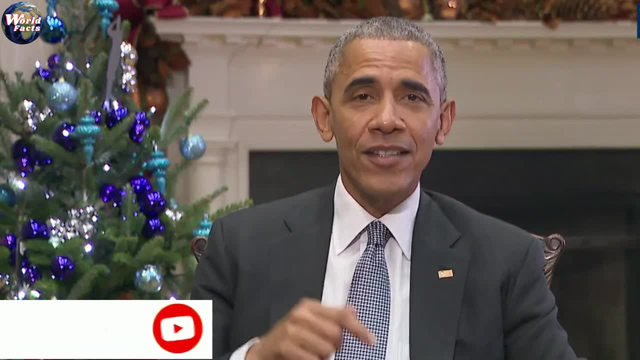 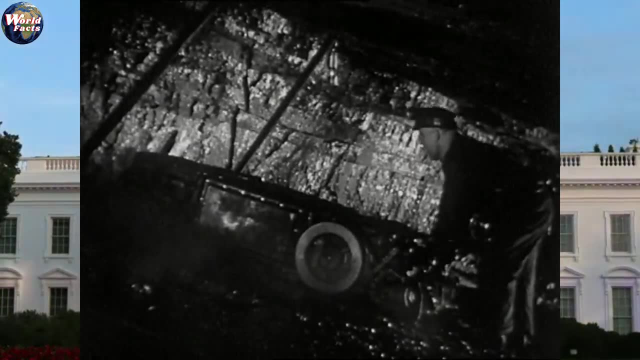 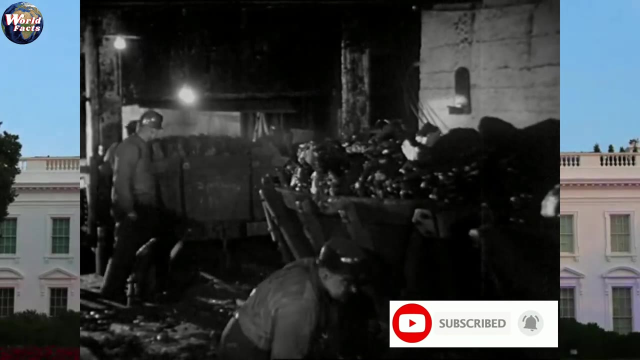 and in 2012 he was re-elected for a second term. the achievements of the past 100 years have made the united states a world leader in economic, military and technology. the united states is the largest coal reserves in the world. it is known as the biggest trading country and heavily